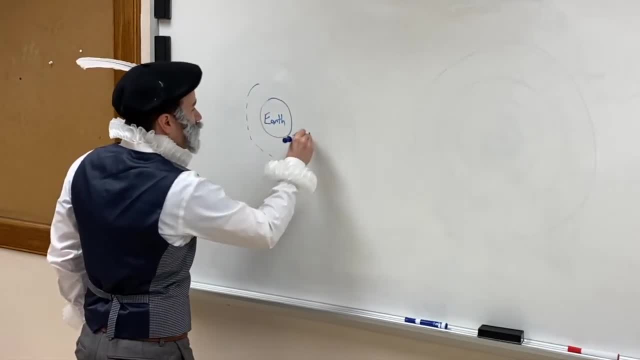 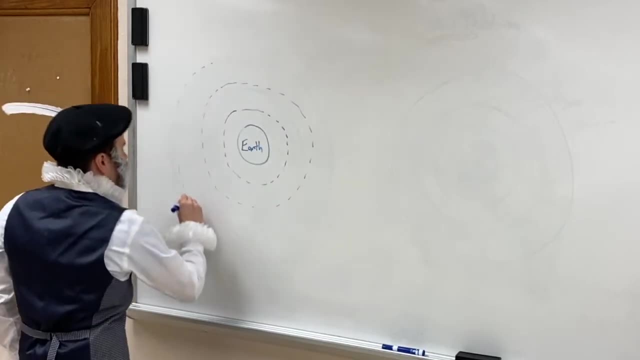 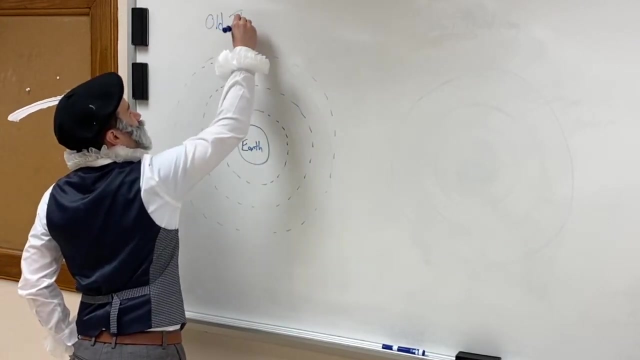 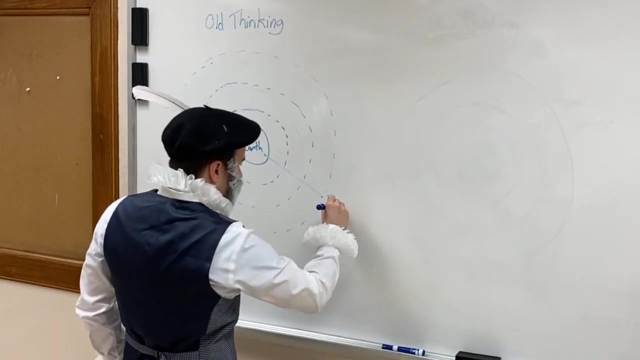 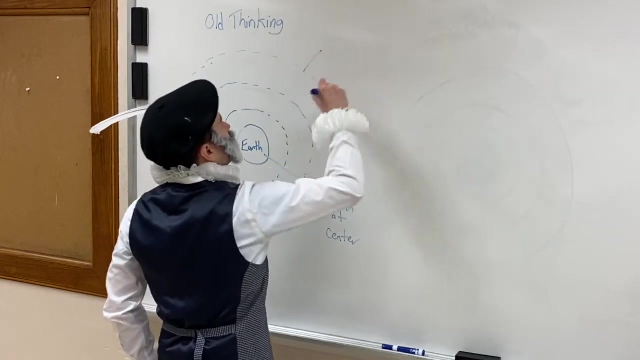 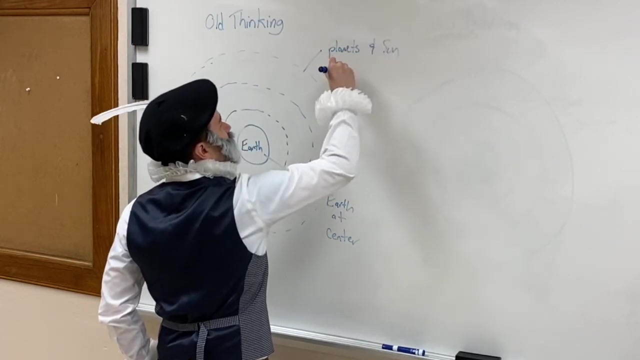 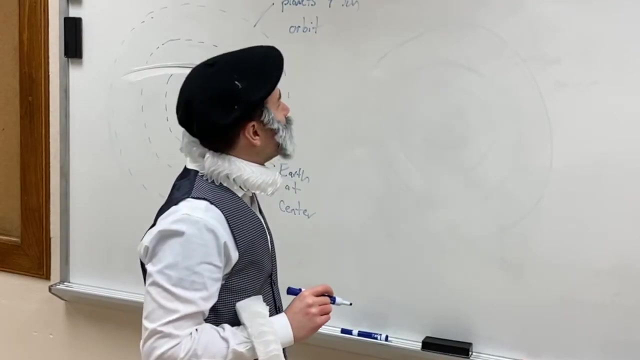 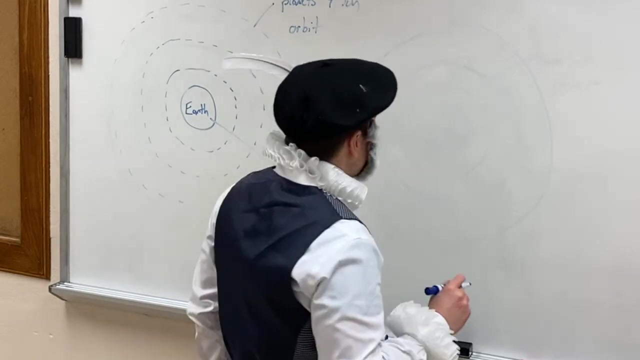 And around us orbit all the celestial objects in perfect circles. Let's call this orbit Old thinking. Notice: here we have Earth at center and planets and sun orbit in perfect circles. Sometime later there was a new thought. Nicholas Copernicus shook things up, shook up the scientific community and proposed: 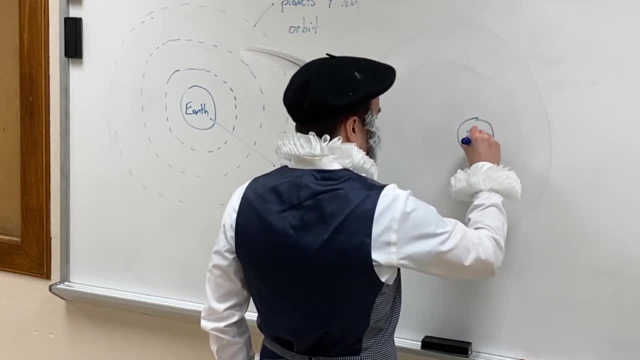 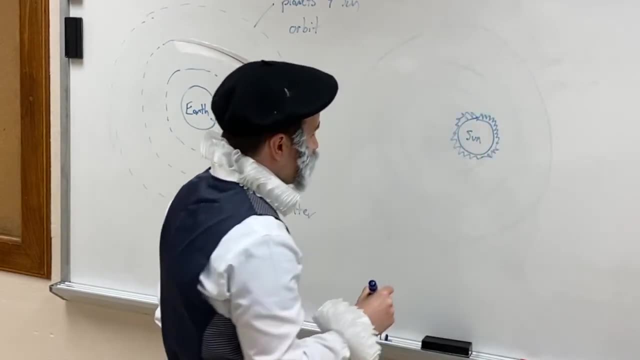 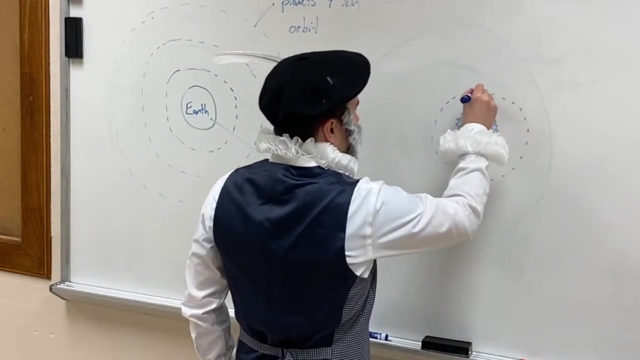 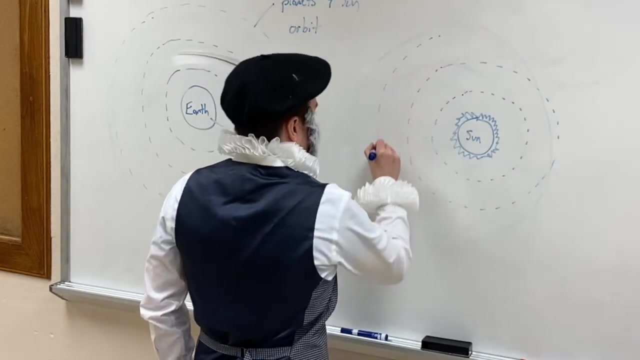 what if we put the sun at the center of the solar system? Let's draw those flames, the hot sun. If the sun lies at the center, then orbiting around it are all the other members: Mercury, Venus, Earth. 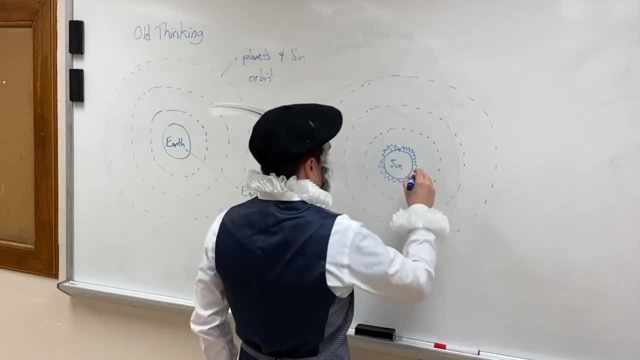 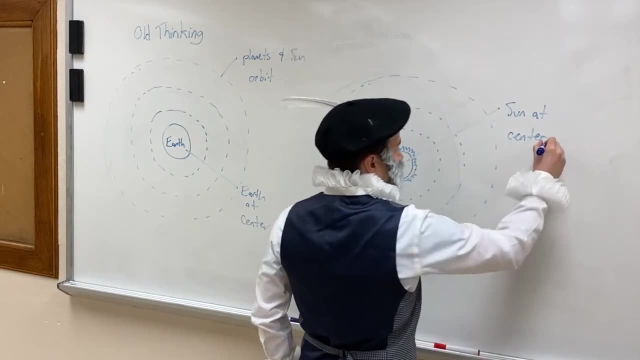 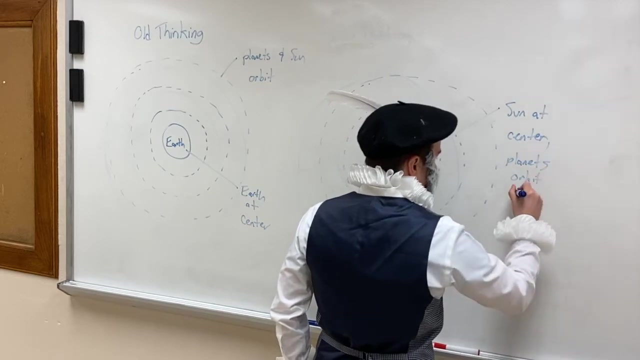 So key components here is sun at center and planets orbit around. The sun is at the center of the solar system and planets orbit around it. The sun is at the center of the solar system and planets orbit around it. So now our demonstration is over. 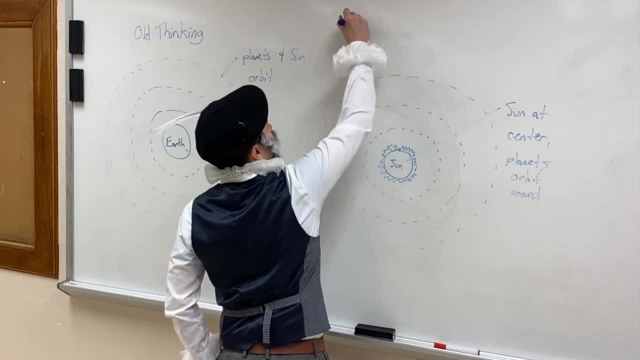 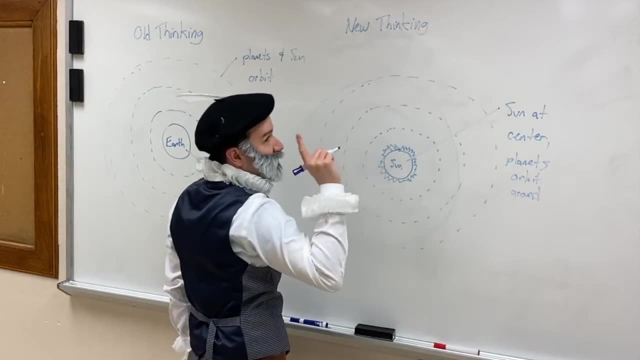 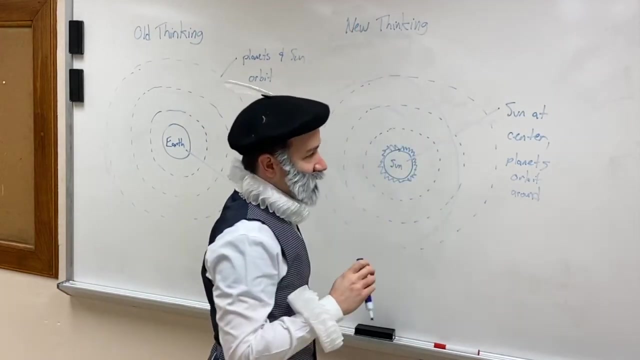 Let's see our first event opportunity when we tried this on Jupiter. Let's call this New Thinking. Now, the new thinking led to results that were pretty good, but still not perfect. There were still errors, So we could not be sure that this was the correct one. 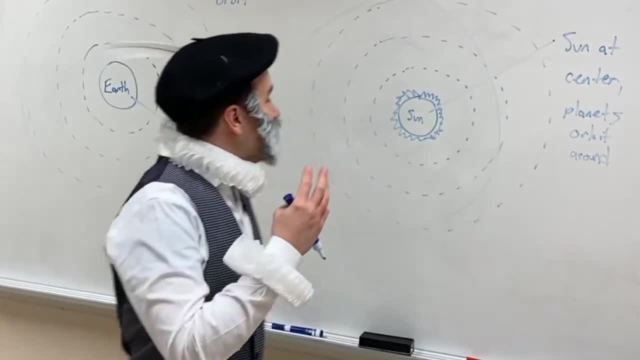 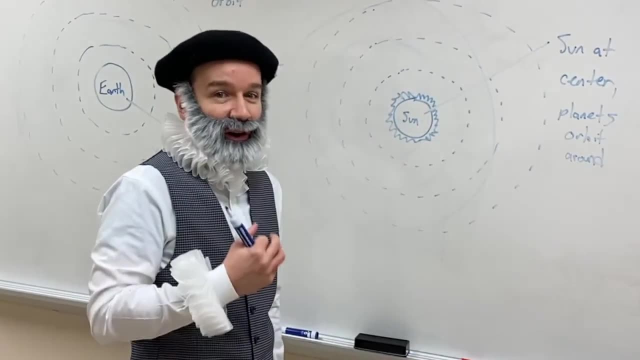 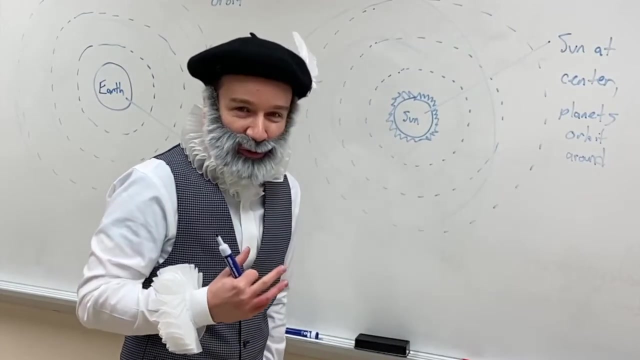 This is where I came in, And I was invested in trying to find out which shape it was and which arrangement that could best adapt it. So I knead these videos together- best described the solar system- On my quest to understand how this arrangement is laid. 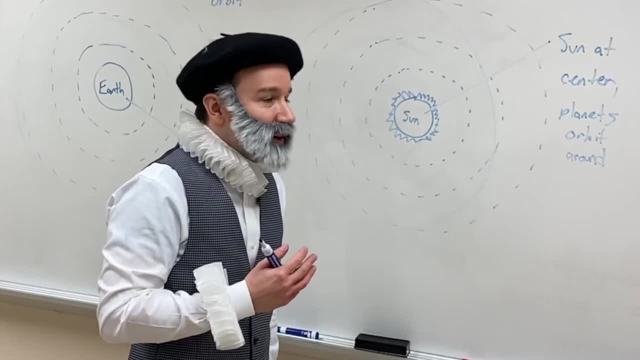 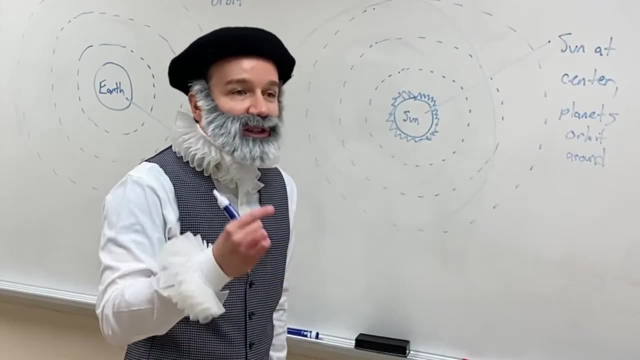 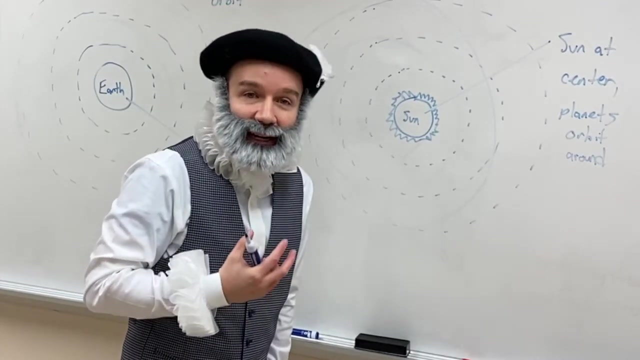 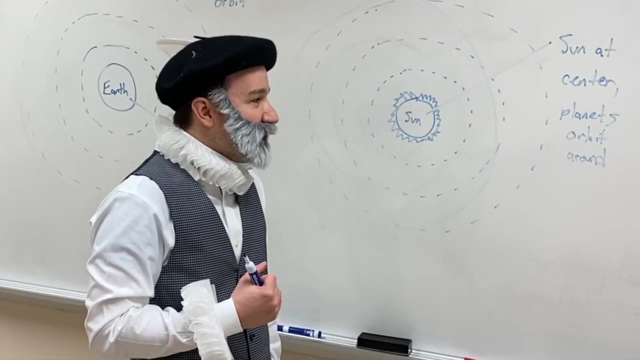 out, I came across the work of Tycho Brahe, who is known across the world for having the best measurements of the positions of the planets over many years, And these are the data that I needed to be able to solve the question that burned in me. I worked hard. 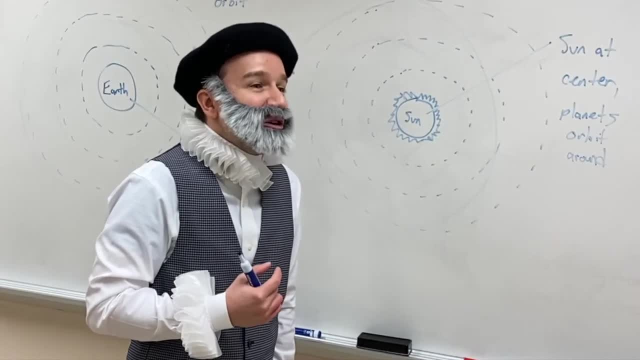 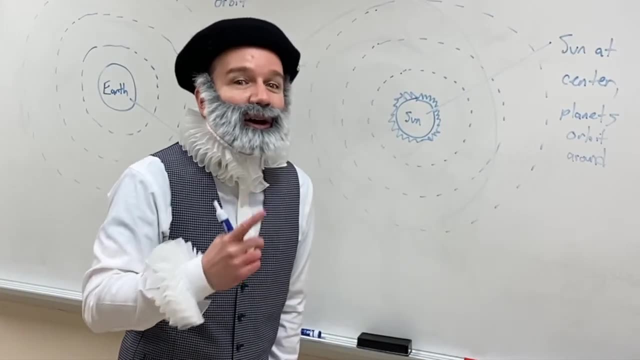 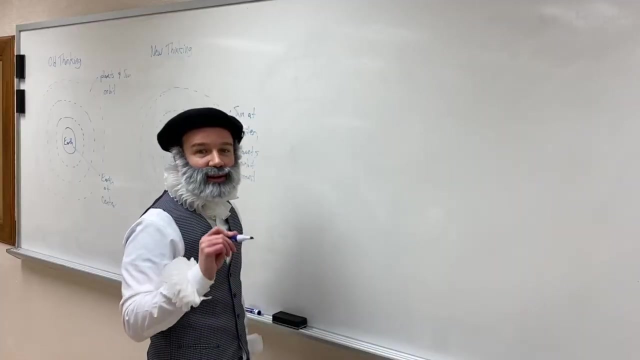 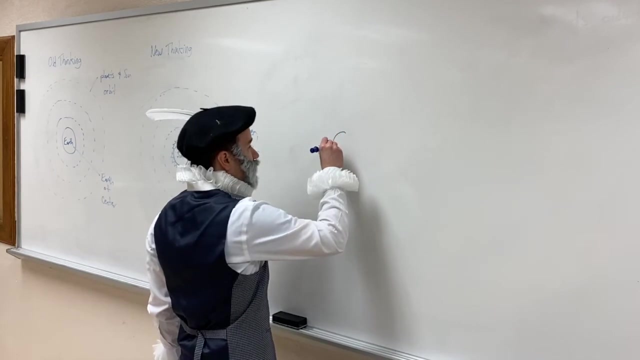 to get a job with Tycho. but Tycho was very suspicious of my intentions because in fact he had hired me to prove his own system that I didn't necessarily believe in. Tycho had his own system. He wanted the Earth to remain at the center of the solar system, But he recognized the 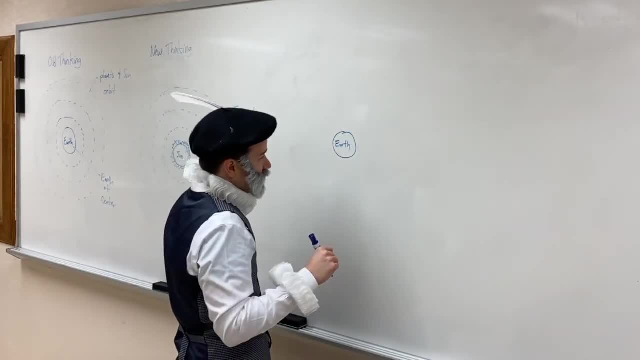 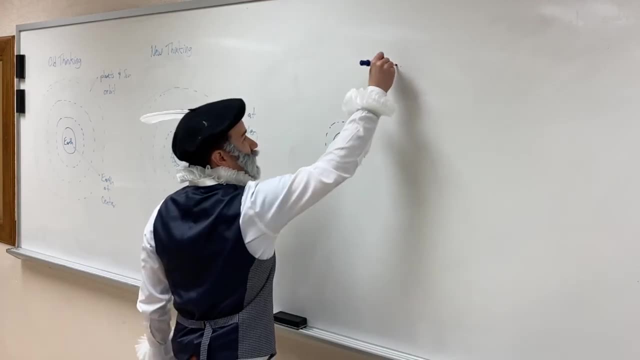 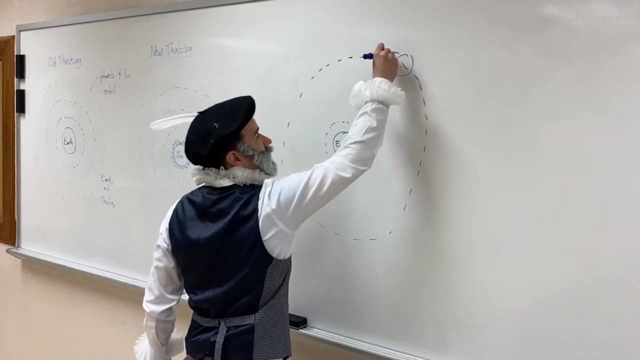 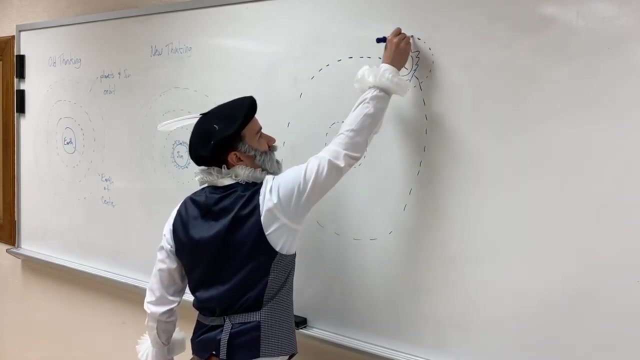 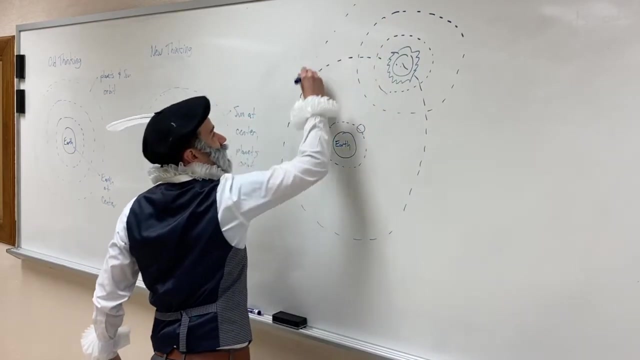 challenges of making all the other planetary bodies orbit around it. So he retained the Moon around the Earth, but then placed the Sun at a distance. And here's the Sun- and such that it orbited around the earth as the other planets orbit around it. so this: 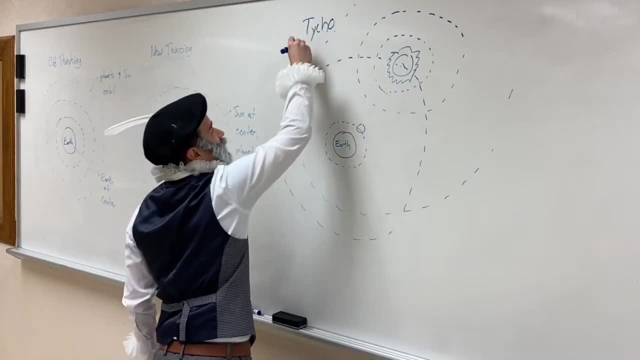 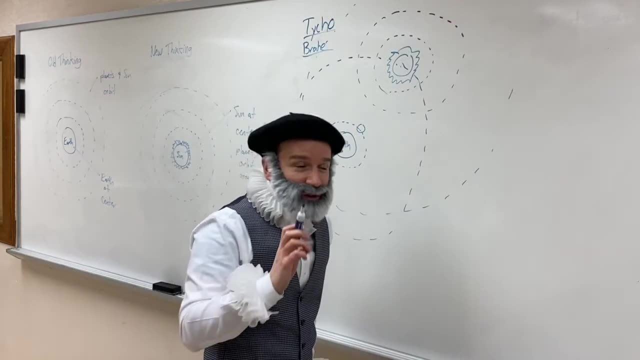 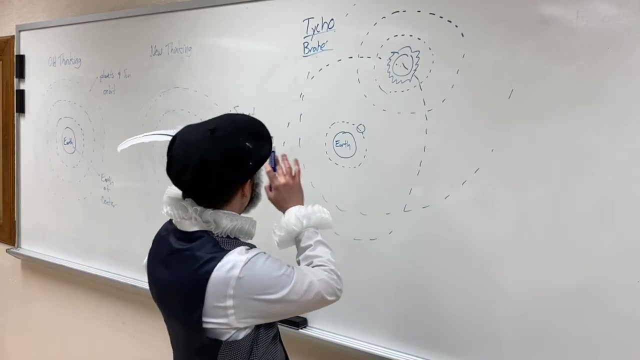 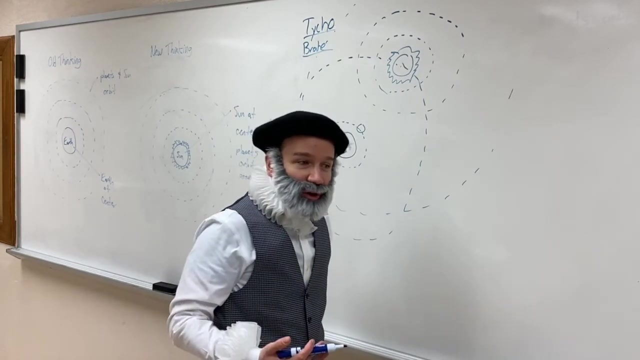 is Tycho Tycho Brahe system. so while I was hired to demonstrate that this was the system, I had suspicions that it was not proper and I wanted to make sure that the other, the new thinking, was the actual, correct one. so I got a job with Tycho Brahe and he slowly gave me observations and I worked at these. 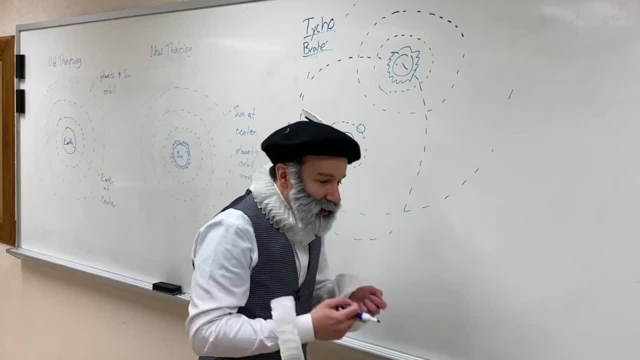 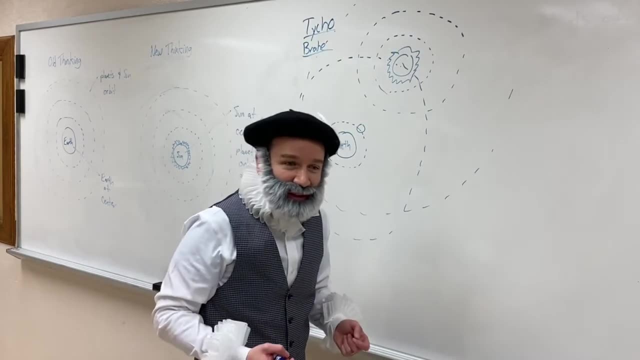 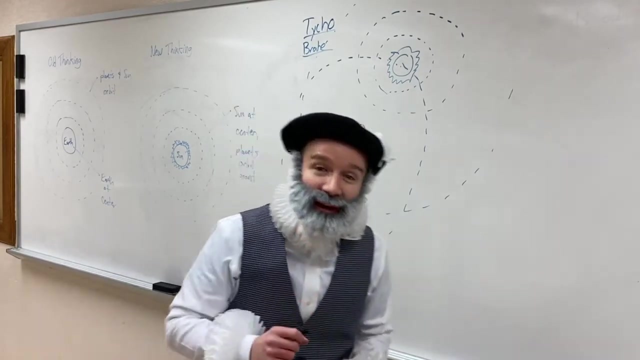 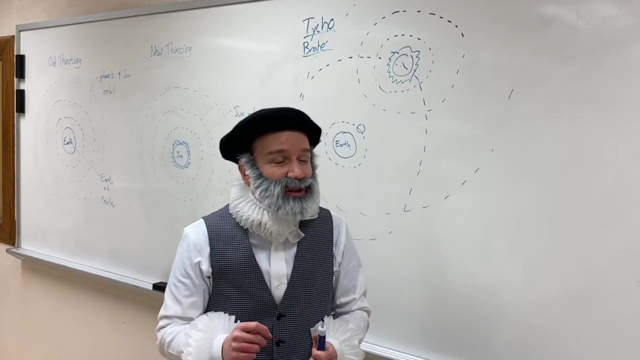 observations day and night to try and come up with the proper calculations. but I needed more. The breakthrough came through with the untimely passing of Tycho Brahe. Some actually were suspicious that I had poisoned Tycho Brahe because it seemed a chance coincidence that I wanted his data and he ended up dying. But 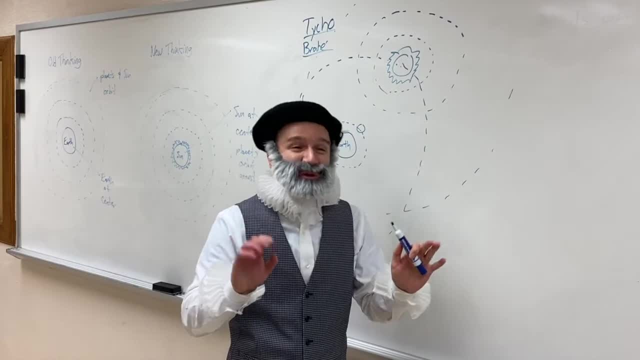 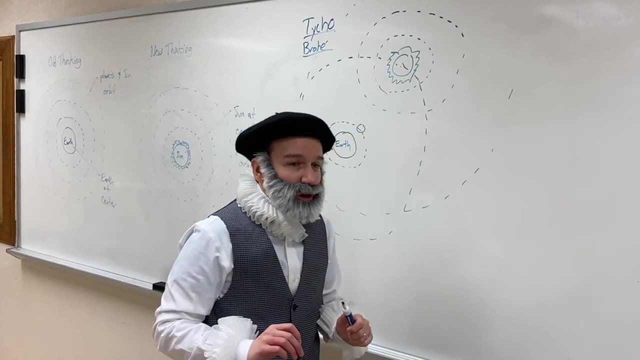 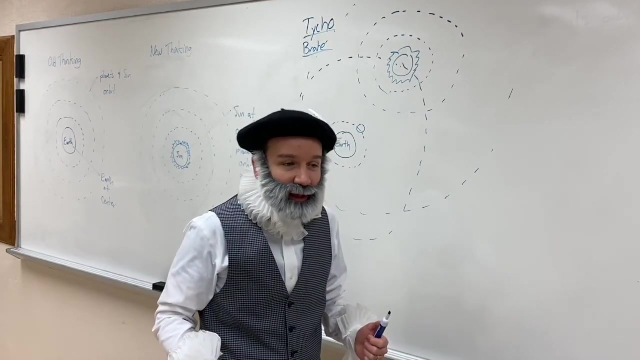 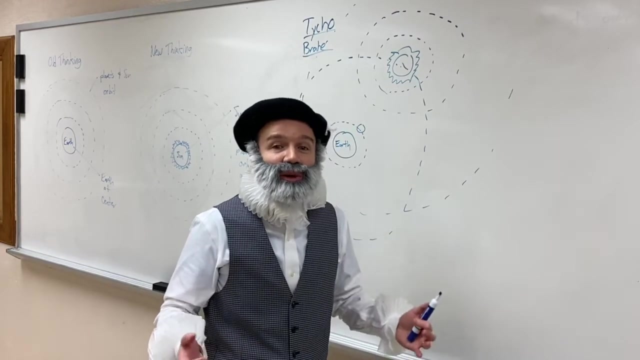 you can read all about it in the news that I was proven by forensic evidence that it was not myself. So there I was, having access to all of Tycho's data, and over 20 years were spent doing all the calculations to determine the laws of planetary motion. These are the laws that you will investigate. 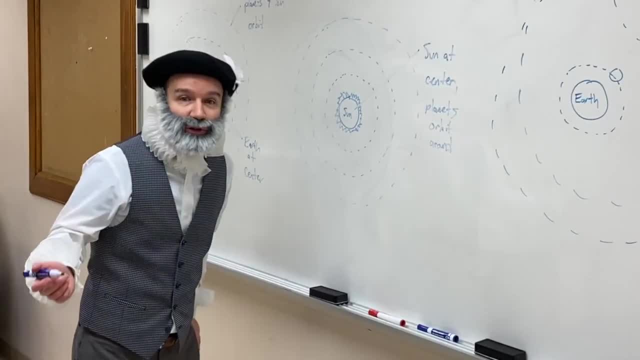 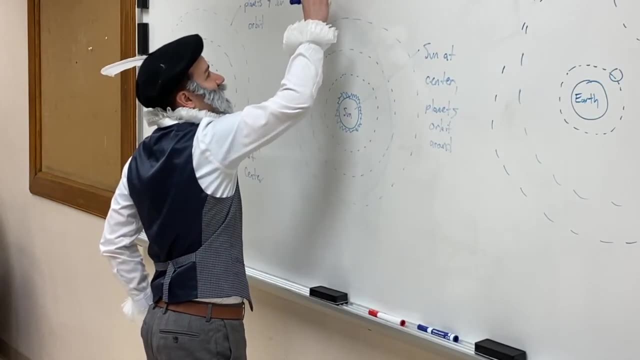 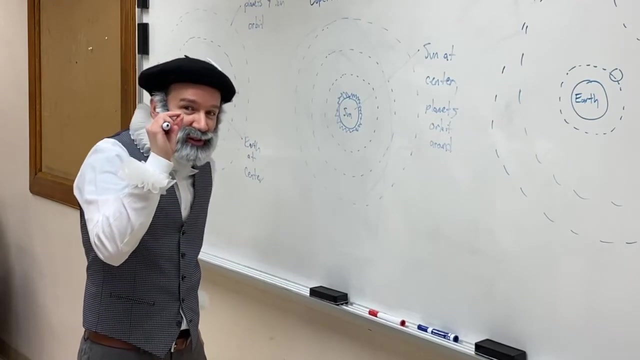 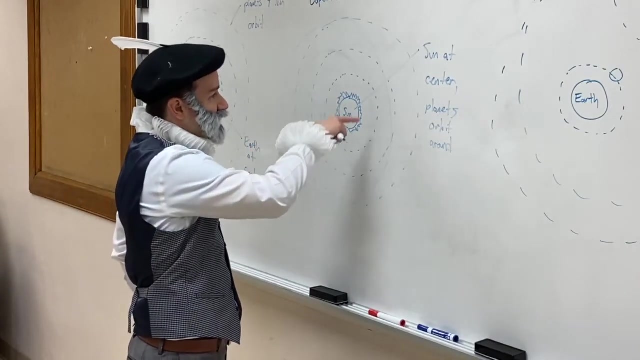 These are the laws that you will investigate. These are the laws that you will investigate. A breakthrough was understanding that this new thinking, contributed by Nicholas Copernicus, had one small but very important detail missing. These were not perfect circles that the planets were orbiting in. They were, in fact. 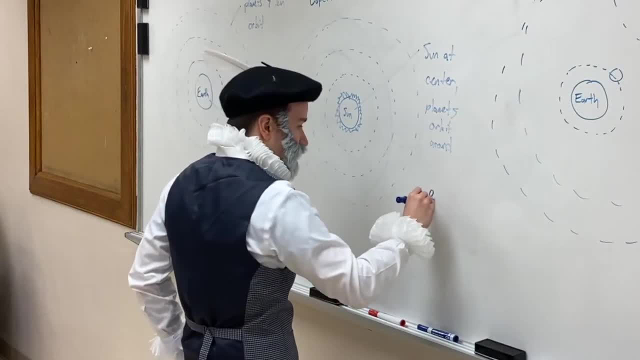 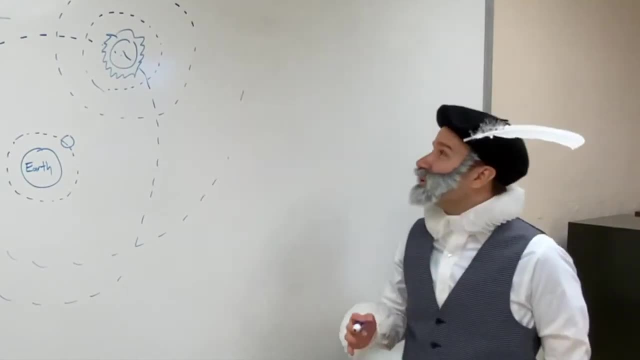 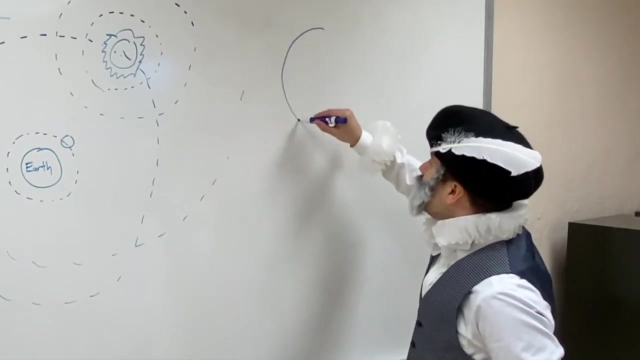 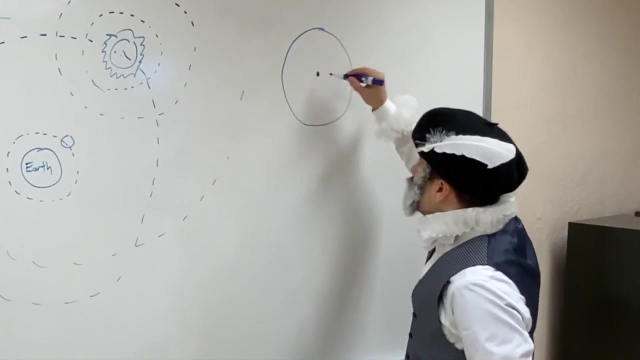 ellipses. Yes, it was an ellipse. Let me describe that a little bit more. I'm sure everyone is familiar with a circle. I'll try to draw a circle as best I can. Circle has one center and from that center, any direction we go out, a certain radius will be the same. 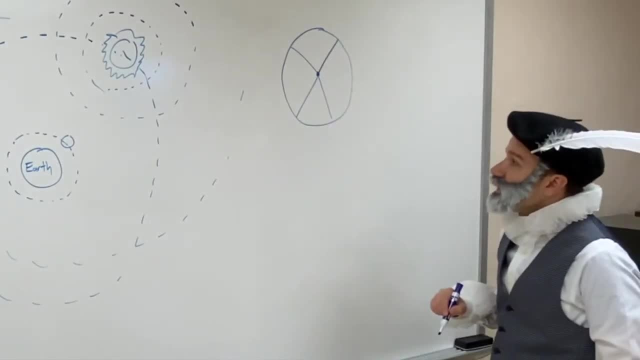 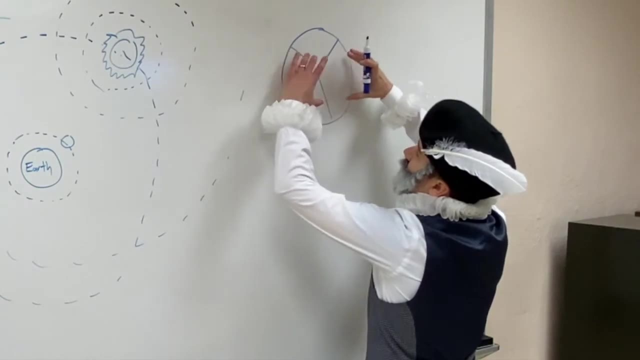 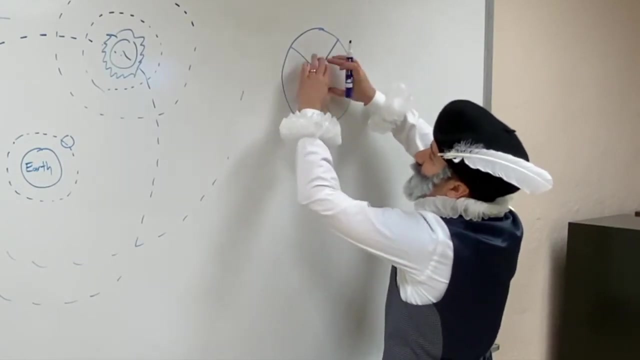 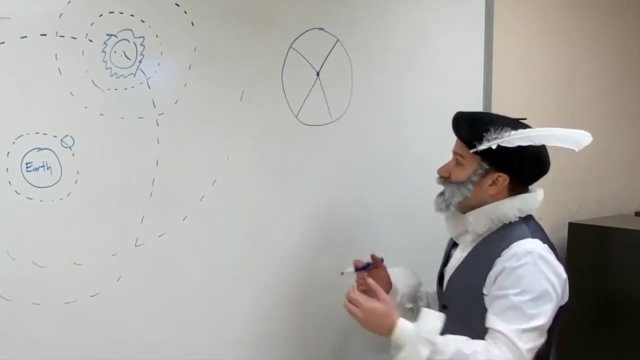 in all directions. In the case of an ellipse, imagine taking that circle and expanding it, stretching it along one axis, So, all of a sudden, that one center becomes two centers, or the language is focuses or foci. Now I will draw the ellipse. 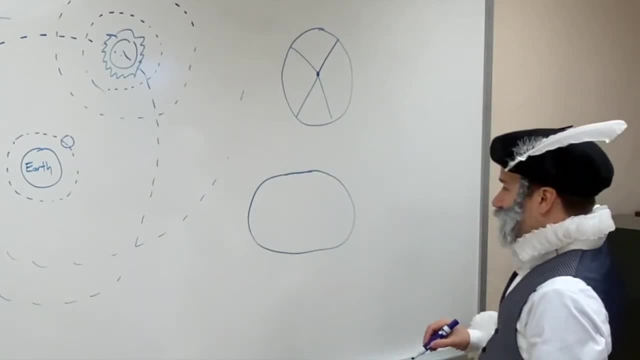 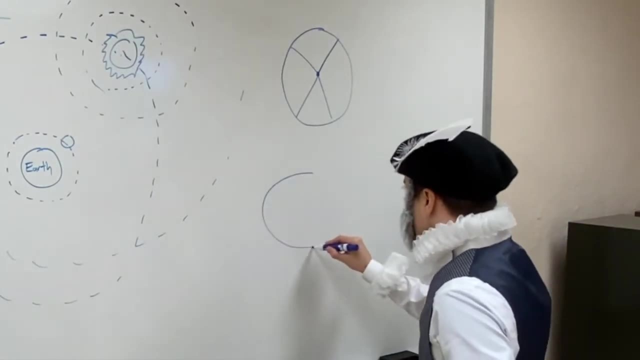 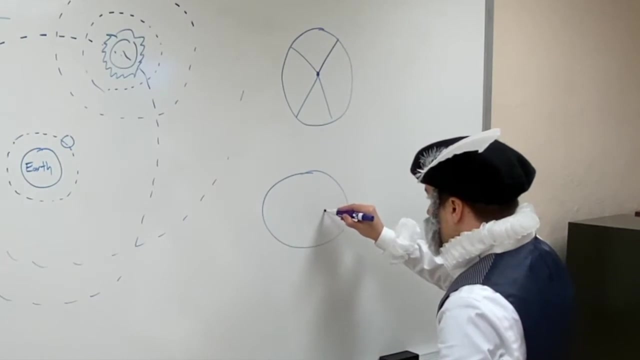 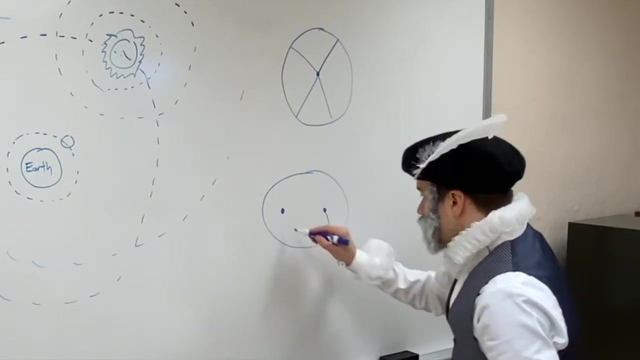 As best I can, and I'm dissatisfied with that ellipse, so I'll try one more time A little bit better. So this center has now been stretched out in two different locations. This is a focus, and this is a focus. I'll call the difference. So this is an ellipse. 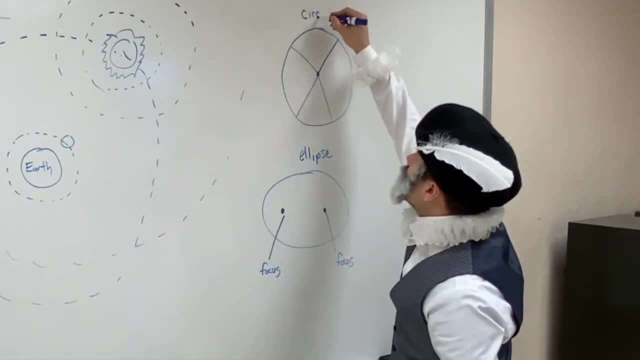 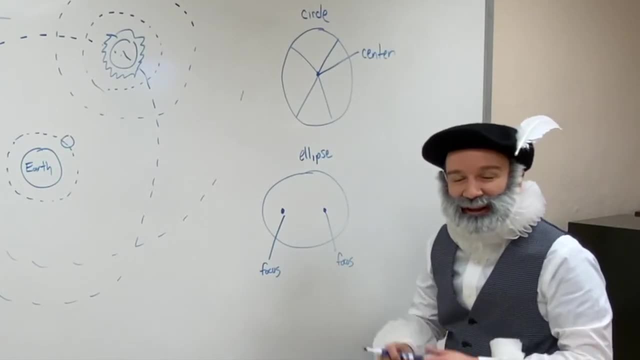 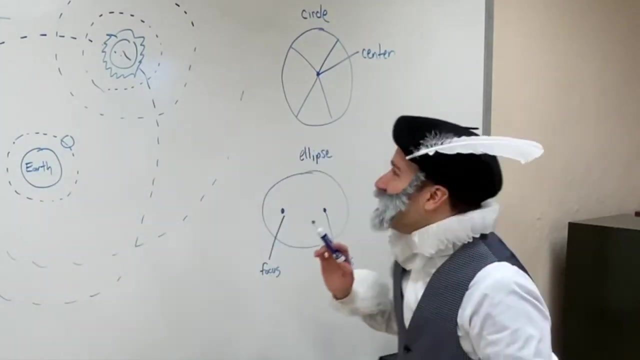 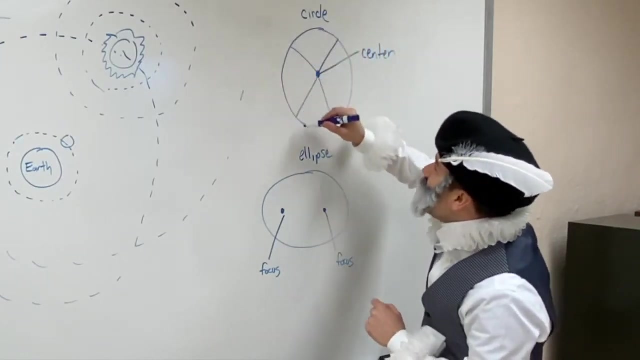 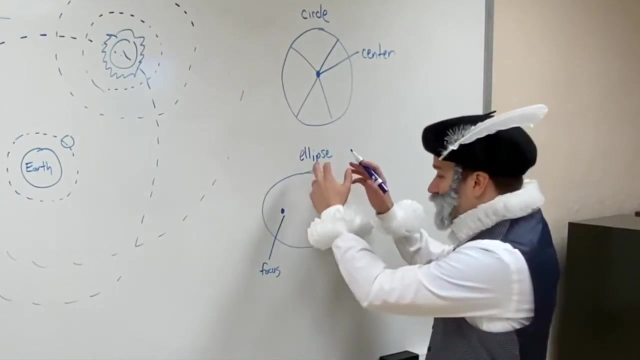 Right, focus, focus. And this is a circle with one center Important to understand what was wrong in the new thinking: They had presumed that sun was at the center and the planets orbited in perfect circles, When in fact they weren't perfect circles, they were ellipses. 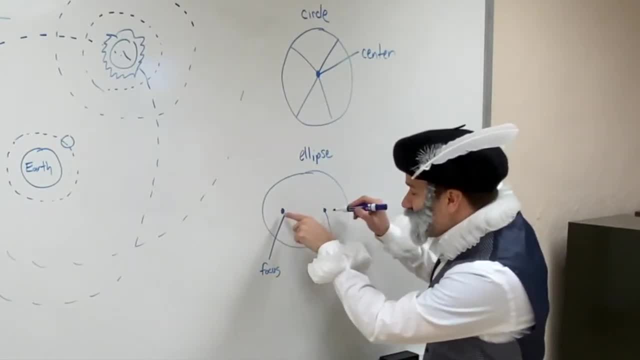 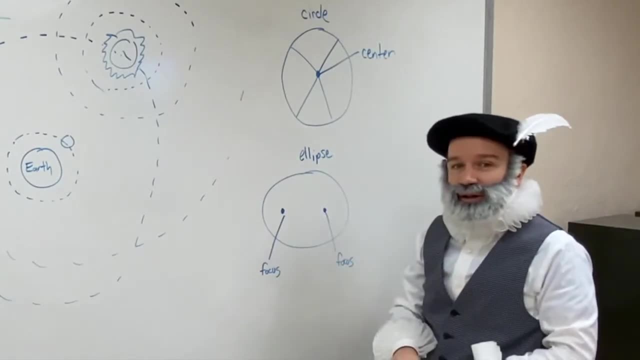 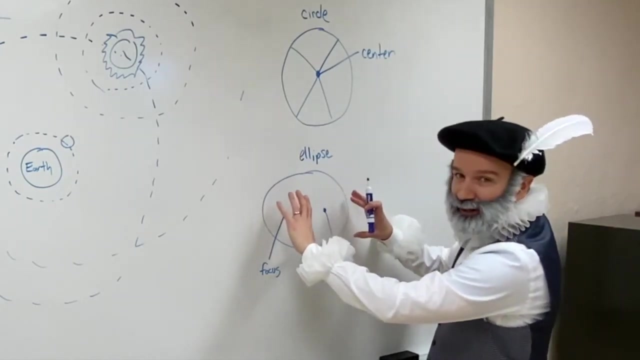 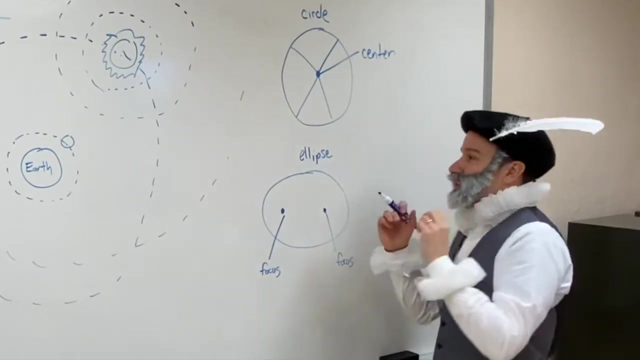 With the sun centered at one of the focuses and the planets following the ellipse around it. Now, in this case, to demonstrate what an ellipse is, I've highly exaggerated the pansed parts of the project. it planets have a very subtle elliptical shape. so if this is an extreme, the orbit. 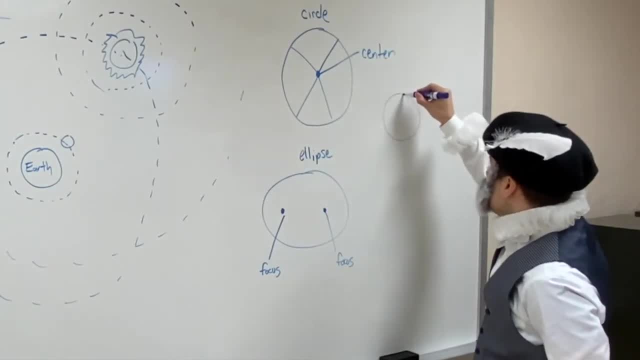 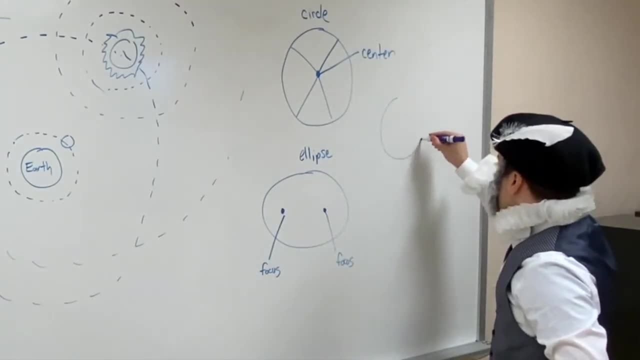 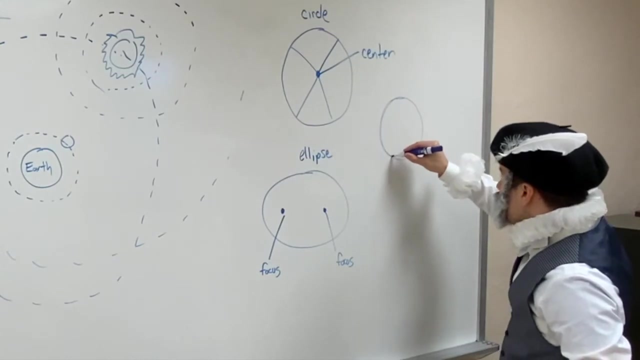 of the planet. if this is a, let's say, a perfect circle, you know the no, that's not a perfect circle. if that is a circle, the ellipticity associated with the planet is going to be just slightly out of whack with that, but it's that small. 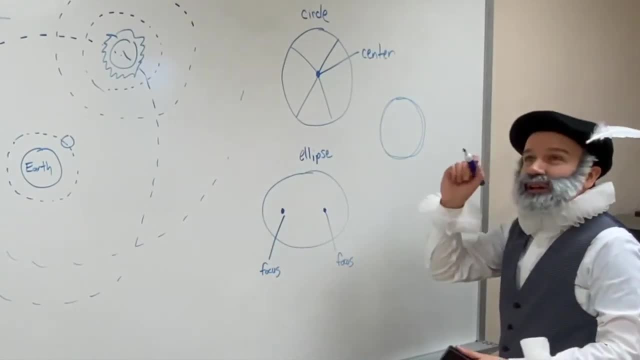 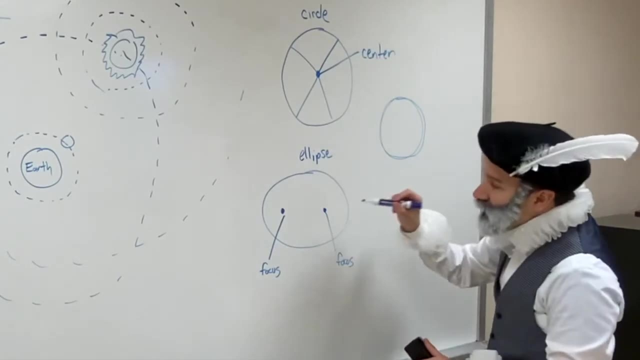 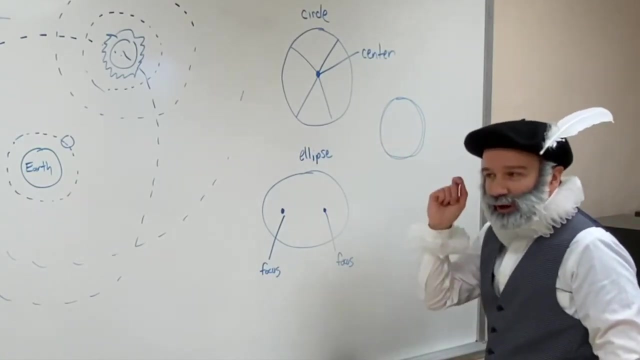 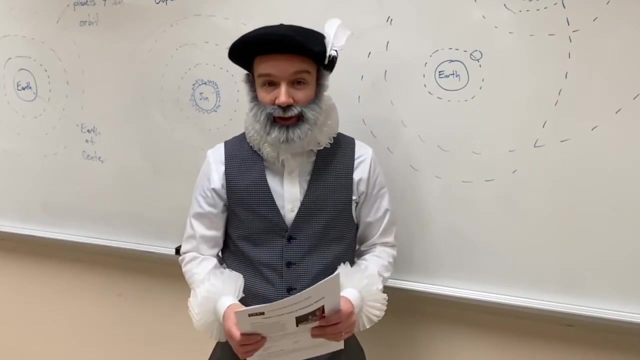 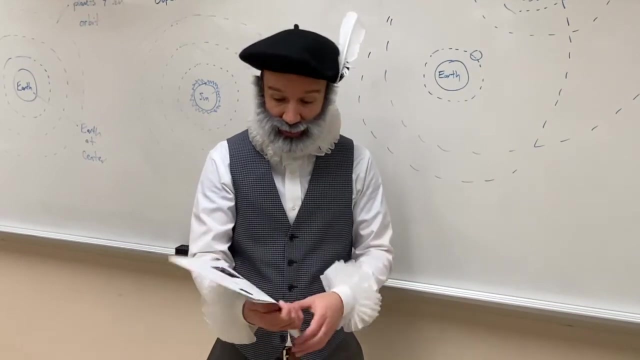 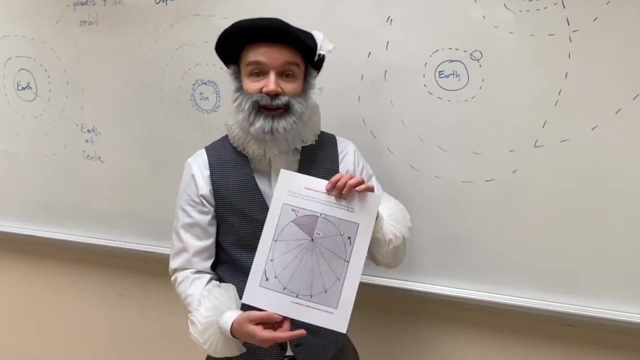 detail. that makes major differences measurable, differences in our predictions of the motions of the planets in the night sky. in making this small adjustment led to superior calculations of planetary motions. and now it's up to you. you have in your hands this activity, which guides you through the process of analyzing data that follows the trajectory of an asteroid. 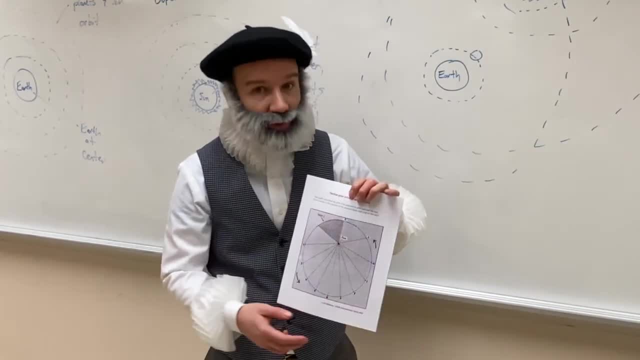 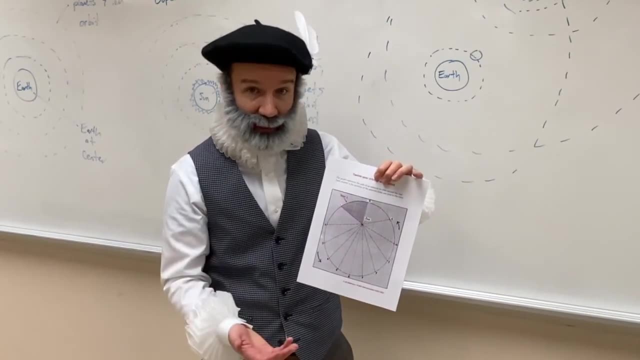 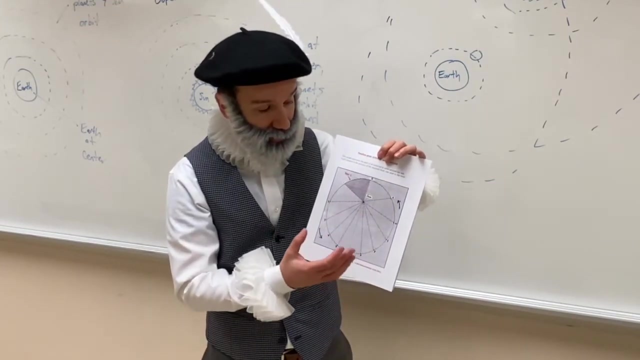 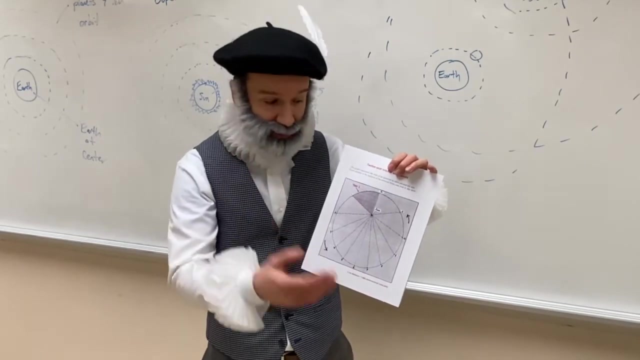 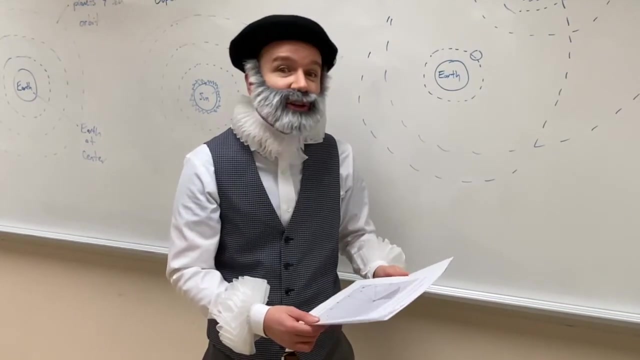 around the Sun. we've chosen an asteroid because its orbit is more elliptical than a typical planet, so the motion is more exaggerated and appropriate. but again, the motions of all the planets are governed by the same planetary orbital motion laws that you will explore through the data. I'll tell you up front that some of this will be. 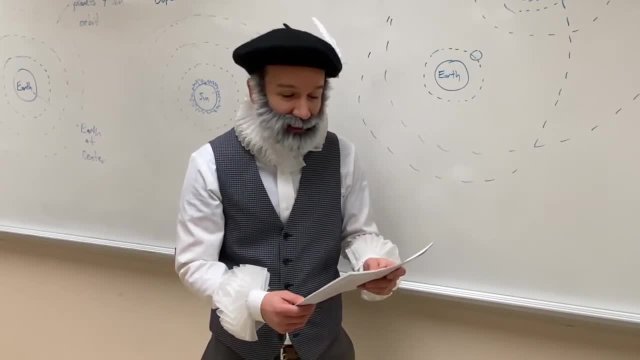 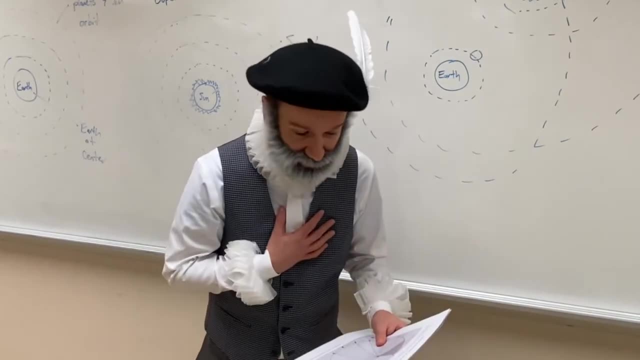 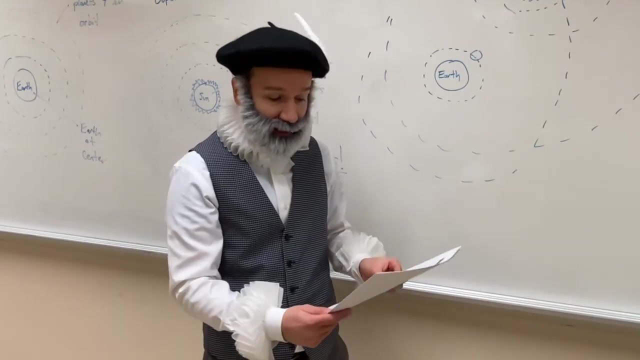 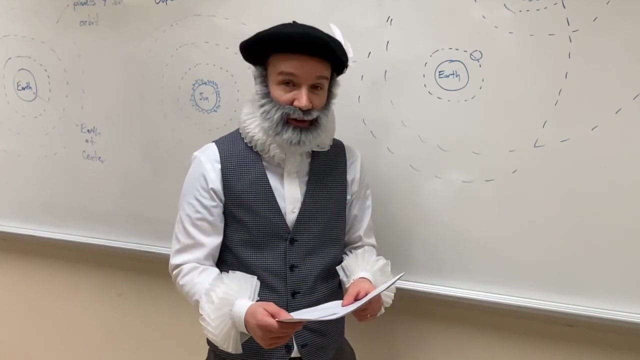 monotonous, and in fact it's meant to be so. I want you to get an appreciation of the type of work that I had to do before I had the luxury of a computer. my hope is that by the end of the activity you will have discovered for yourself the other two planetary laws of motion I've shown.